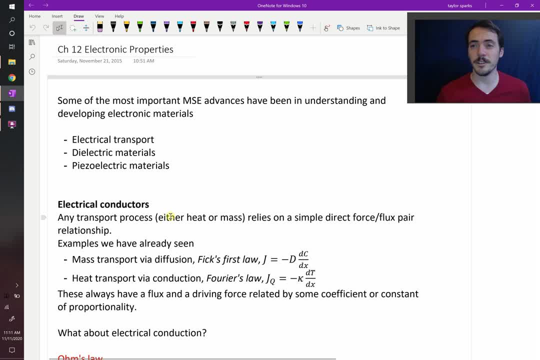 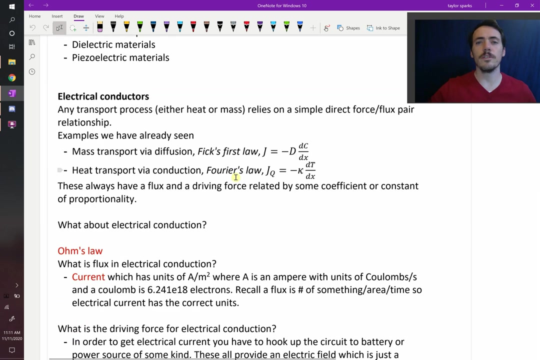 All right, we've reached the chapter on electronic properties of solids in material science And, to be honest, this is one of the coolest chapters, because some of the most fascinating phenomenon and some of the best paying jobs are involved with electronic properties of materials. So we're going to study electrical transport, We're going to study dielectric materials, We're going to study piezoelectric materials, And that's really. there's so much more we could cover, but that's what we're going to do this in this class because it's an introduction. So let's start with this idea of electrical conductors, right? So in any previous transport process, right? 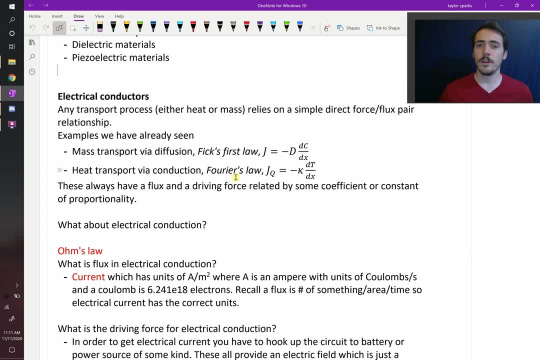 Whether that was transport of heat or transport of mass. what did we have? We always had a very simple relationship, right, We had something that was a driving force and then we had a constant of proportionality that told you how much flux you got in response to that driving force. So remember, in mass transport we called that fixed first law, right For steady state mass transport, where the flux of mass that would be observed is proportional to a constant proportionality, which was called our diffusion coefficient, multiplied by our driving force, which was the gradient in the constant. 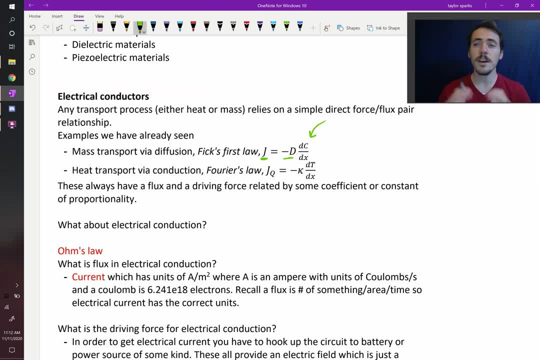 Right, The difference in the composition. Then the same exact thing for thermal transport: right. When there's a flux of heat, JQ, it's going to be proportional to a new constant- This time it's going to be thermal conductivity, and then the driving force is going to be DTDX. right, Our thermal gradient. right. So there's always a flux that's happening in response to a driving force. right, With some sort of coefficient or constant of proportionality. 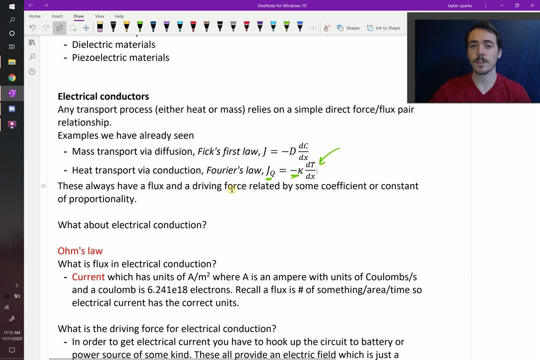 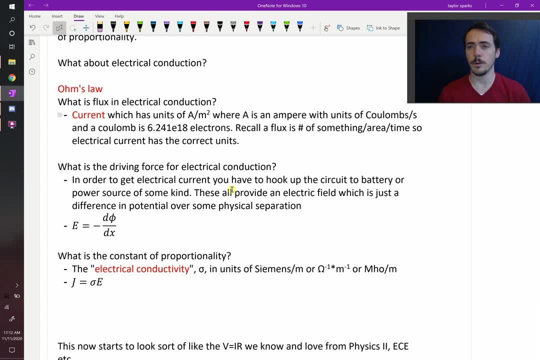 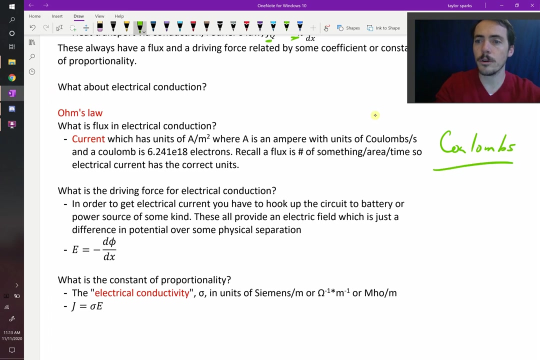 And it's the exact same thing. And it's the exact same thing with electrical conduction. You learned about this in high school, probably in physics. It's called Ohm's Law, right? So, first off, what is the flux going to be for electrical transport? Well, the flux is going to be. our current Current has units of amperes per meter squared right Where an ampere is going to be the units of coulombs per second. So you can see why this is a flux: because we're talking about the amount of something that's going to be coulombs per meter squared. 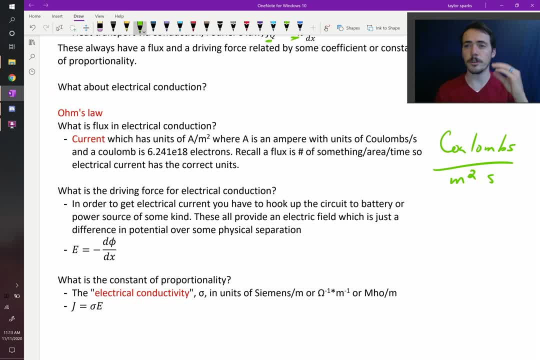 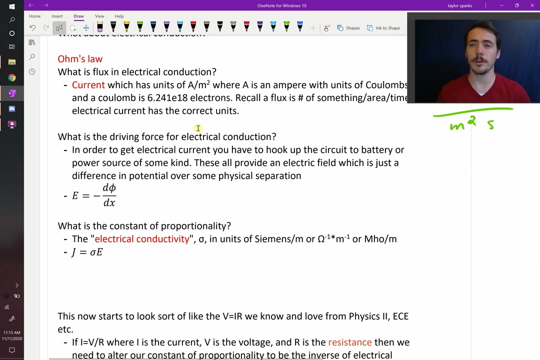 Meter squared per second right. Therefore, it's the amount of something per area per time. So it's a flux. okay, And remember that a coulomb is just equal to some number of electrons: 6.241 e to the 18 electrons. okay, So we know that this is a flux. When we talk about current, this is now a flux. So what's going to be the driving force? Well, we say here that in order to get electrical current, you have to hook the circuit up to a battery or some sort of power source, And these all provide an electric field. right, An electric field. 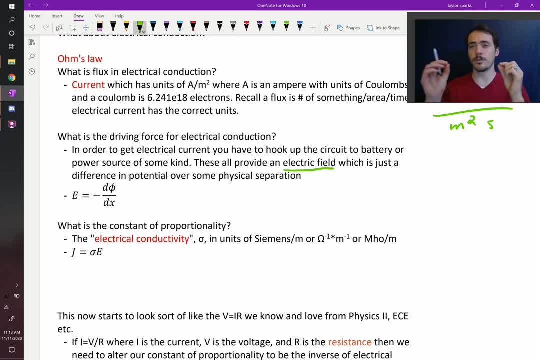 An electric field And that's really just a difference in the potential across something, right? So if I have this pen here and I apply a battery, you know I connect battery terminals to either side of this, since the battery has a voltage. by connecting it to either end of this, I induce a voltage, right, A difference in potential across this object, right? So that's what this is. E is our electric field. That's just equal to the difference in the potential, the electrostatic potential, divided by the distance, right? So if this is, you know, 6 inches long and there's a 9 volt distance across it, we can calculate. 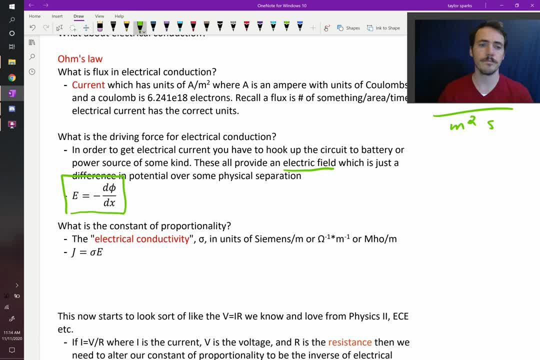 the electric field. It's going to be 9 volts divided by that 6 inches. right, So we have our flux, We have our driving force. Now we just need to know what the constant of proportionality is, And that is going to be the electrical conductivity. right, It will have the units of siemens per meter. Sometimes we call that inverse ohms per meter, Or we sometimes even call it mows per meter, which is mow is ohm written backwards. I didn't come up with these, That's just what's out there, right? 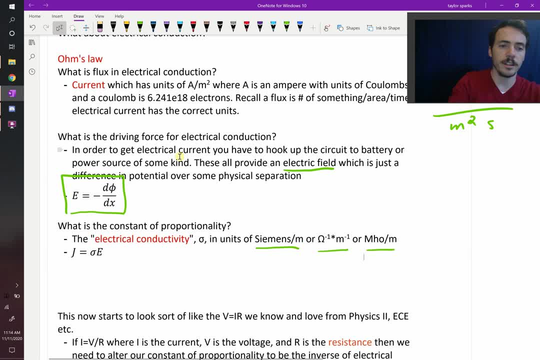 They're all the same thing. So that allows us to write, finally, our Ohm's law. We have J, our flux. This is electrical flux, right? So current is going to be equal to our conductivity multiplied by our electric field. So this doesn't quite look like V equals IR. It's getting closer, right? Remember Ohm's law: V equals IR. We're not quite there, even if we rearranged it, So we need to change it just a little bit. Well, if we write it with 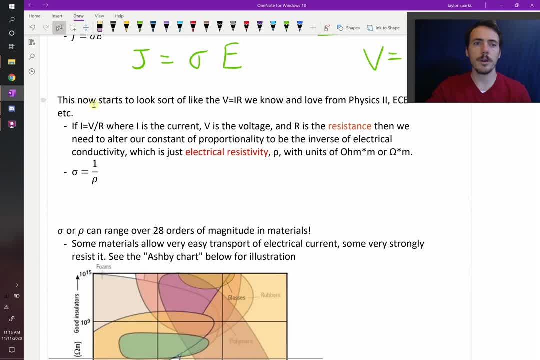 I equals V over R. that's getting closer, right. But it's V divided by R, not V, which we're substituting for electrostatic potential, electric field. right, We know that V, the voltage, is going to actually be the electric field, because you have to take into account the geometry of your 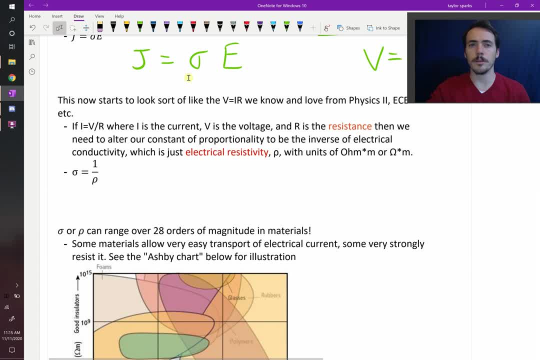 sample, But you're also dividing it by resistance rather than multiplying it by conductance. So that's fine. We can talk about electrical this constant of proportionality for electrical transport. in either terms of conductivity or resistivity, It's equivalent One. 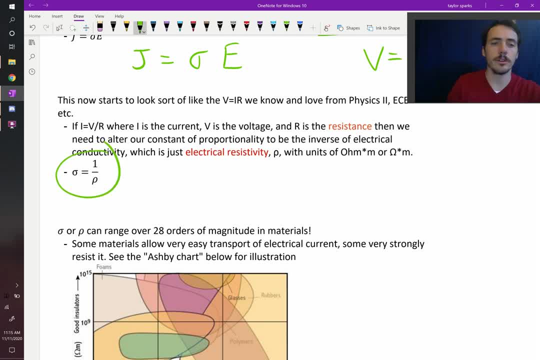 is one over the other right. Our electrical conductivity right here is equal to one over our electrical resistivity, and vice versa. So it doesn't matter, You can talk about it in either scenario. It just switches the units Instead of what were our units before, it was inverse Ohms. 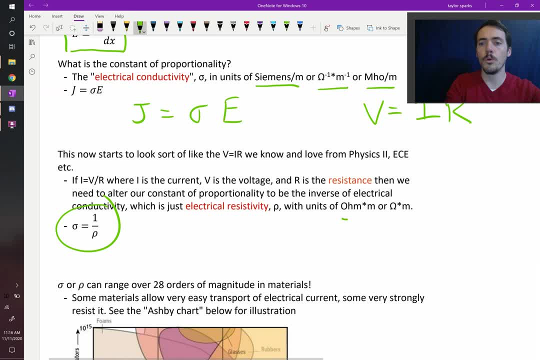 per meter. Well, now, when we take one over that, the units are going to be Ohm meters. right, That's the most common way to represent this. okay, So that is our electrical conductivity and our electrical resistivity. And what's amazing to me, 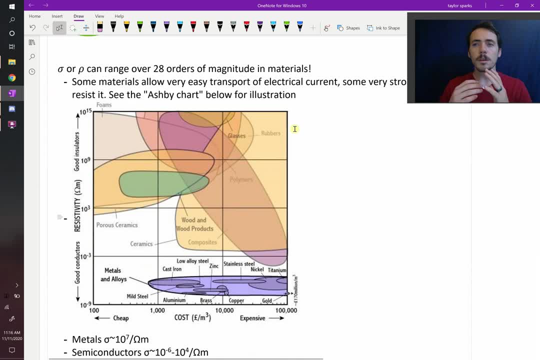 is. if you look at these plots that show material properties for lots and lots of different classes of materials, we see that electrical conductivity it can change over 28 orders of magnitude, Massive differences in the ability of a material to conduct electrons or not at all. right, So this: 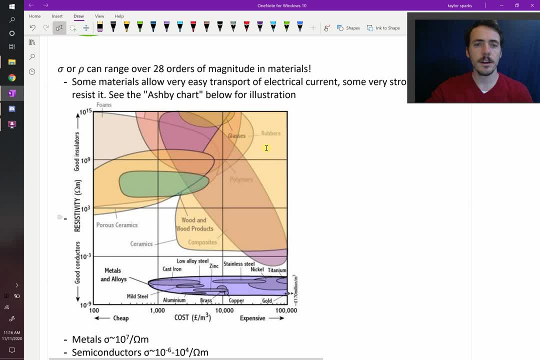 is called an Ashby plot, from Michael Ashby, the guy who came up with these. Here you see a bunch of different classes of materials: wood, polymers, glasses, rubbers, metals- all these different things- And on the y-axis, look what they have plotted. 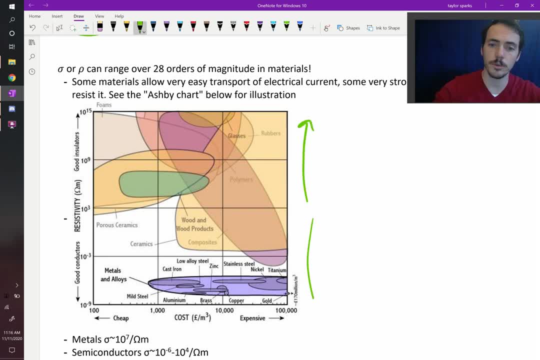 And on the bottom you've got resistivity. So up here these things are really good insulators, and as you move down you've got good conductors. so things like metals And again you span from something like 10 to the 15th Ohm meters- very, very resistive, all the way down to. 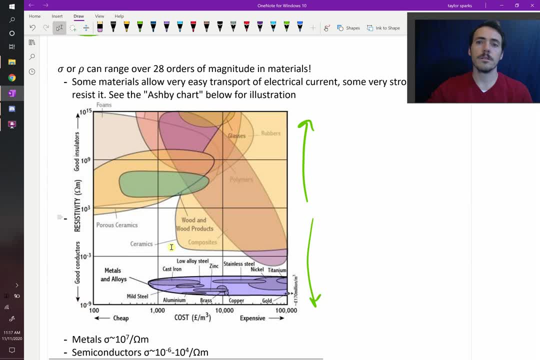 10 to the negative ninth Ohm meters, so extremely conductive. So there's a huge, huge, ginormous, maybe the biggest of any material property difference in the material property. So why, So why? What's going on here? 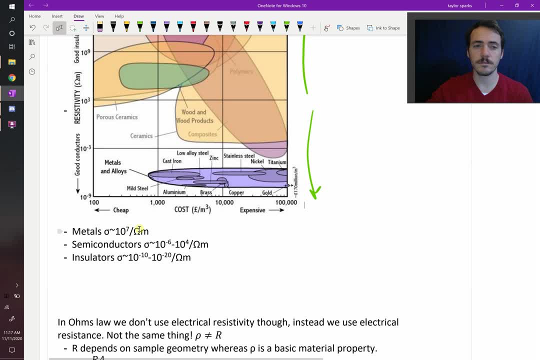 Just some typical values. Metals typically have a conductivity right. We're switching back to units of conductivity instead of resistivity, But the conductivity of metals is something like 10 to the 7th per ohm meter. Semiconductors are something like 10 to the minus 6th, all the way up to 10 to the 4th. 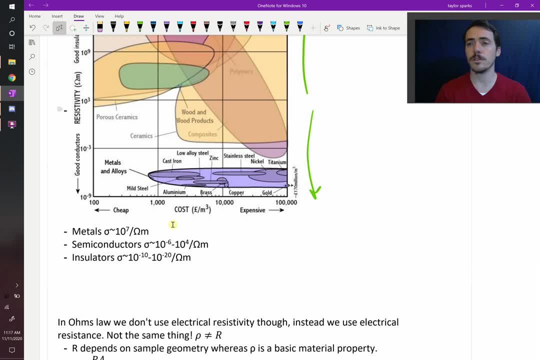 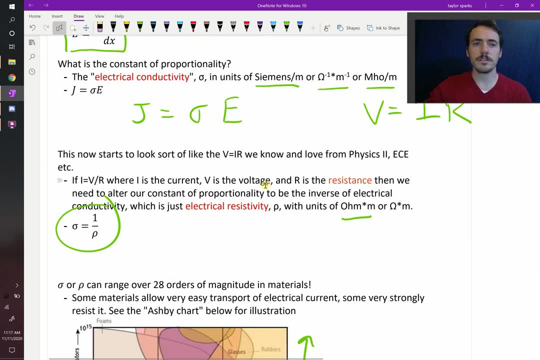 so they can vary pretty widely. And then insulators- things that don't conduct electricity, are typically like 10 to the minus, 10 to the 10 to the negative, 20 per ohm meter. okay, Okay, so we now have something that's looking a little bit closer to Ohm's Law, right? 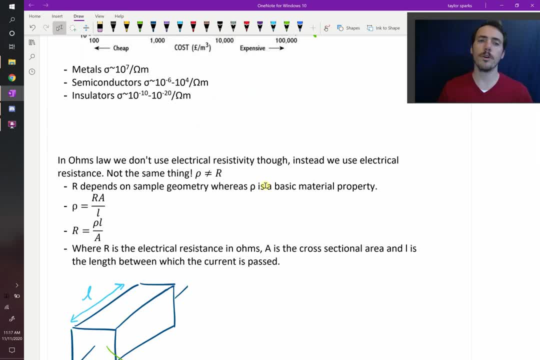 But there is one last thing we need to cover here, and that's the fact that with Ohm's Law, we're not using resistivity, We're using overall resistance, And- this is a key thing to note- that resistivity is not the same as total resistance.